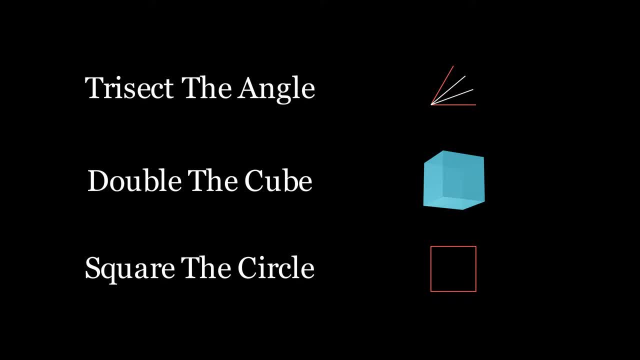 Now you might ask yourself: why would this be so hard? It sounds pretty easy to me, And you would be right. They do sound pretty easy. So easy, in fact, that a third grader might even attempt it. But I can assure you you. 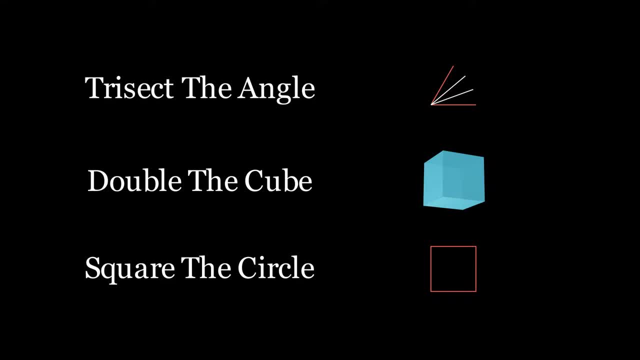 too, would only waste your time trying to come up with a solution. And spoiler alert, that's because there is none. In fact, it has long been proven that a solution to any of these problems does not exist. But before we really get into these three interesting problems, I want to make sure 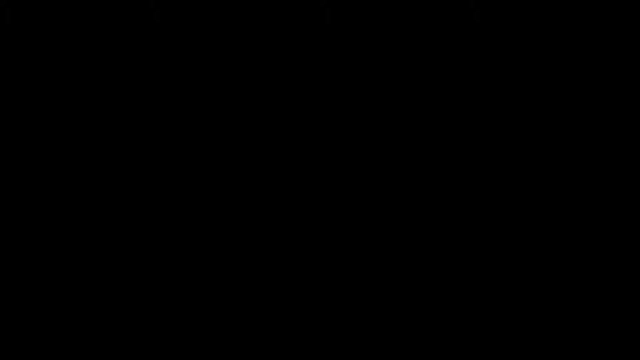 that we're all on the same page when it comes to geometry and constructions. In a construction, we can only use a compass and a straight edge to make a figure or shape With a compass. we can only use a compass and a straight edge to make a figure or shape With a compass. 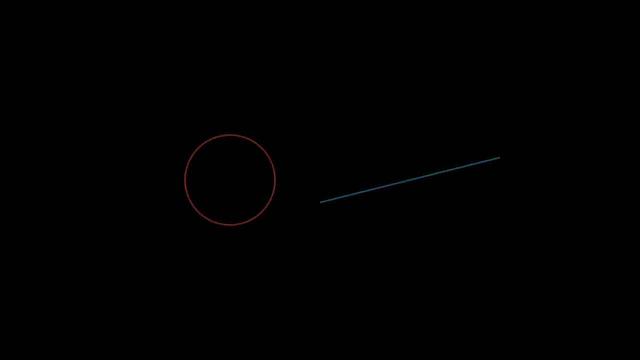 you can make circles, And with a straight edge you can make straight lines, And that's it. You might think this is pretty limited, but these tools are actually quite powerful. If we're given a unit segment, then we, through geometry, are physically able to add, subtract. 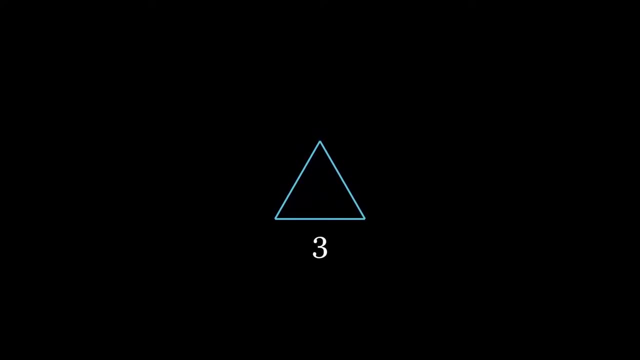 multiply, divide and even take square roots of rational numbers. This is important because it allows us to transform a difficult geometrical problem into an algebraic problem, giving us more to work with. An important distinction in these constructions is that we're not given a ruler, but instead a straight edge, something without markings. 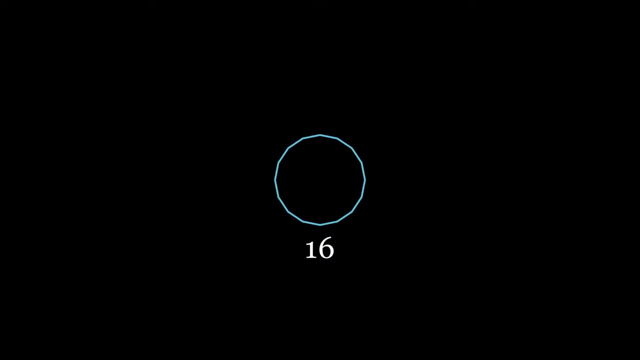 You might be excited to know that if we did have a ruler, all of these problems would have easy, simple solutions. But that's not the case here and it's one of the reasons these problems are so hard. But enough of that, Let's get into our first problem: trisecting the angle. 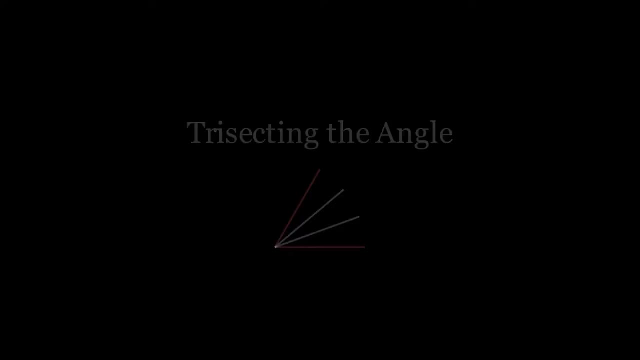 I think we can all agree that a 90 degree angle can easily be trisected. Just construct an equilateral triangle to see why. However, what we want to show is that not every angle can be trisected. To demonstrate this, all we have to do is find at least one angle that can't be trisected. 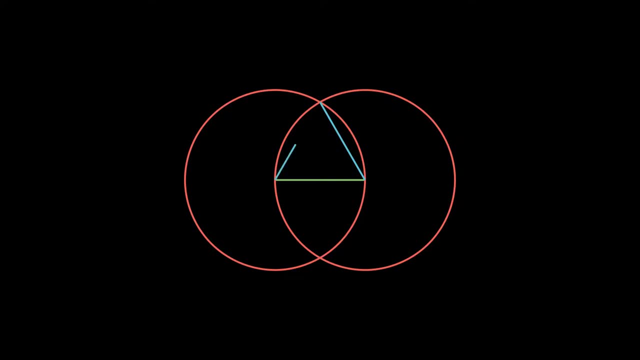 If we're given a unit segment, then we, through geometry, are physically able to add, subtract, multiply, divide and even take square roots of rational numbers. This is important because it allows us to transform a difficult geometrical problem into an algebraic problem, giving us more to work with. An important distinction in these: 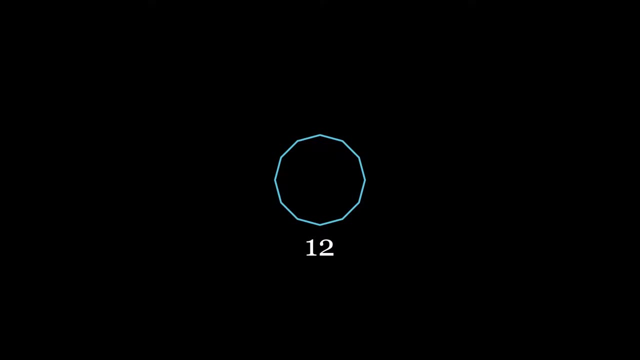 constructions is that we're not given a ruler, but instead a straight edge, something without markings. You might be excited to know that if we did have a ruler, all of these problems would have easy, simple solutions. But that's not the case here, and it's one of the reasons these problems are so hard. 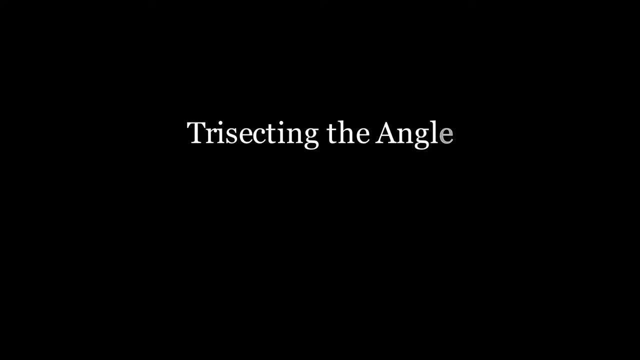 But enough of that, Let's get into our first problem: trisecting the angle. I think we can all agree that a 90 degree angle can easily be trisected. Just construct an equilateral triangle to see why. However, what we want to show is that not every angle can be. 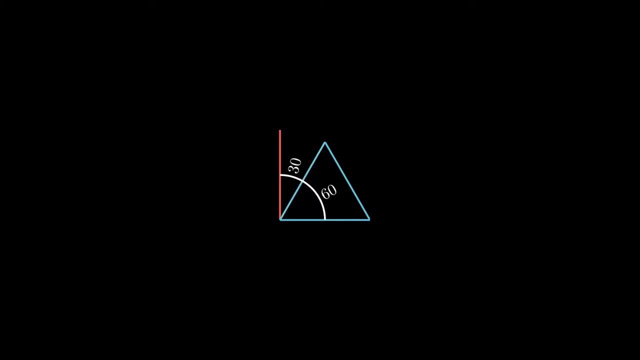 trisected. To demonstrate this, all we have to do is find at least one angle that can't be trisected with compass and straight edge. To start, I'll demonstrate how we can construct an arbitrary angle in the familiar Cartesian plane. Given some angle, theta, all you need to do to construct it. 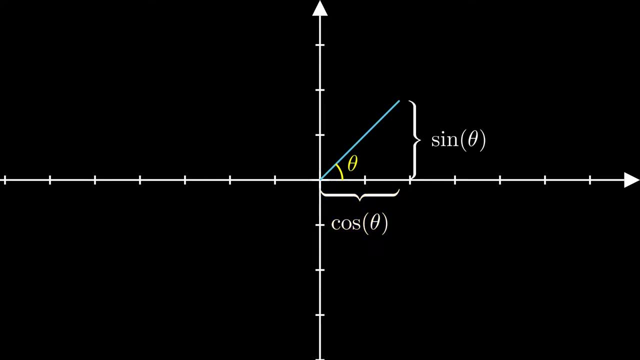 is, construct the cosine of theta and the sine of theta, as these are just the x and y coordinates of the angle. So if cosine of theta is constructable, it follows that the angle is constructable too, and vice versa. Now suppose we have a 60 degree angle. 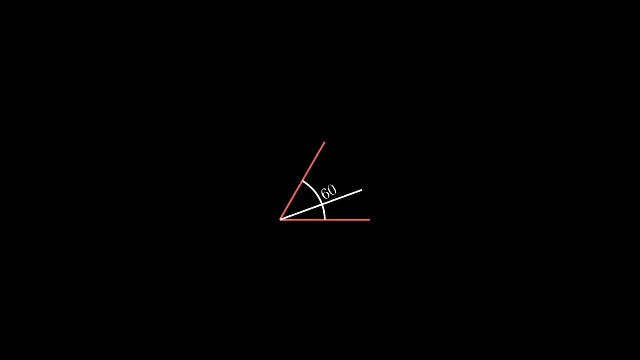 We want to find out whether or not we can trisect it. If we can trisect a 60 degree angle, then that means that we can construct a 20 degree angle and in turn, the number cosine of 20 degrees is constructable. There's a handy trigonometric formula which, at the moment, 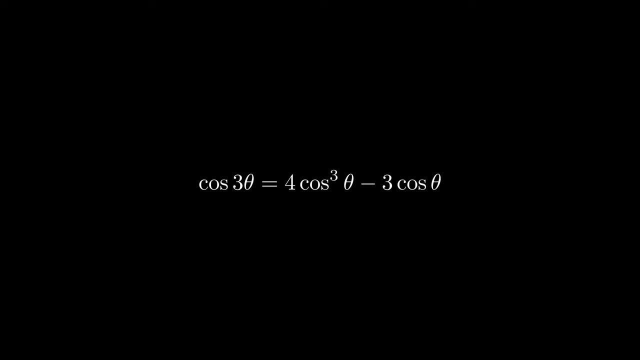 looks unnecessary and strange but in the end helps us solve our problem. If we let theta equal 20 degrees and substitute x for cosine of 20 degrees, then what we're left with is a polynomial with cosine of 20 degrees as a root. Furthermore, 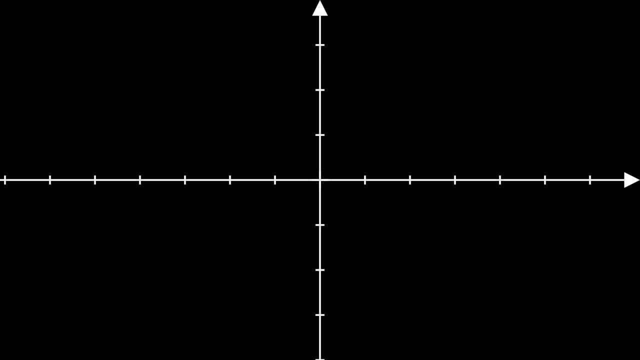 with compass and straight edge. To start, I'll demonstrate how we can construct an arbitrary angle in the familiar Cartesian plane. Given some angle theta, all you need to do to construct it is construct the cosine of theta and the sine of theta, as these are just the x and y coordinates. 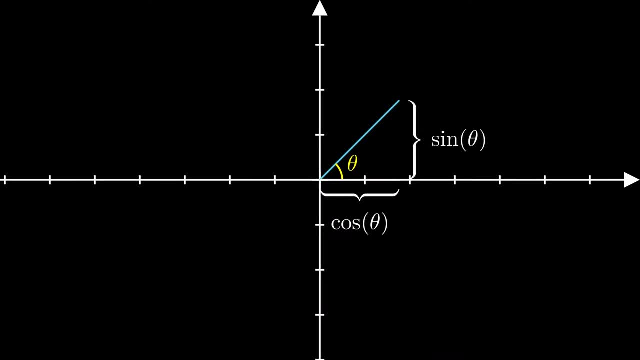 of the angle. So if cosine of theta is constructable, it follows that the angle is constructable too, and vice versa. Now suppose we have a 60 degree angle. We want to find out whether or not we can trisect it. If we can trisect a 60 degree angle, 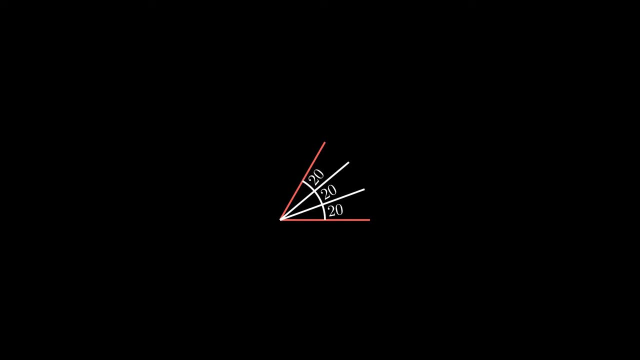 then that means that we can construct a 20 degree angle and in turn the number cosine of 20 degrees is constructable. There's a handy trigonometric formula which at the moment looks unnecessary and strange but in the end helps us solve our problem. 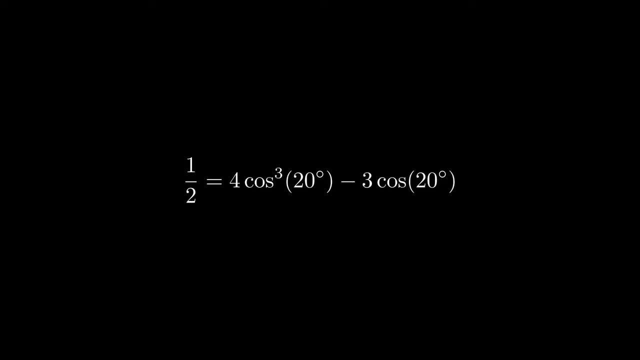 If we let theta equal 20 degrees and substitute x for cosine of 20 degrees, then what we're left with is a polynomial with cosine of 20 degrees as a root. Furthermore, I'll substitute 2x for y, which will help us out in a bit. 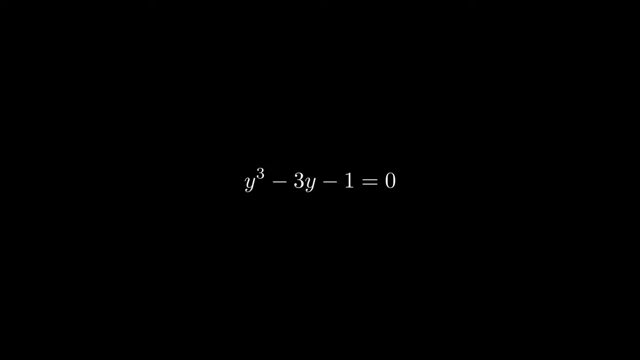 At this point you might be asking yourself where we go from here. This is where abstract algebra comes in. Basically, any root to our polynomial is not constructable if we can't factor it with rational numbers, and its degree is not a power of 2.. 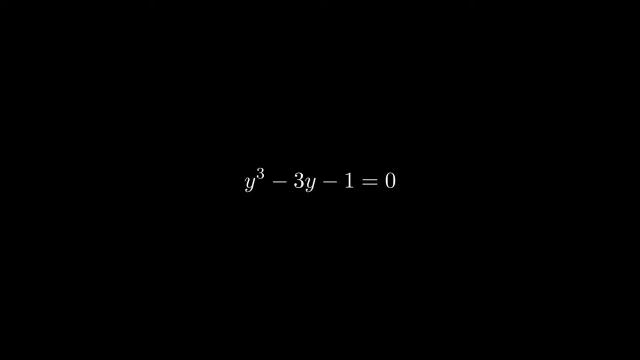 To check whether this polynomial is factorable with rational numbers, all we have to do is use the rational root theorem. Our constant term is negative 1, and our leading coefficient is positive 1, so our only possible roots are positive 1 and negative 1.. Some quick mental. 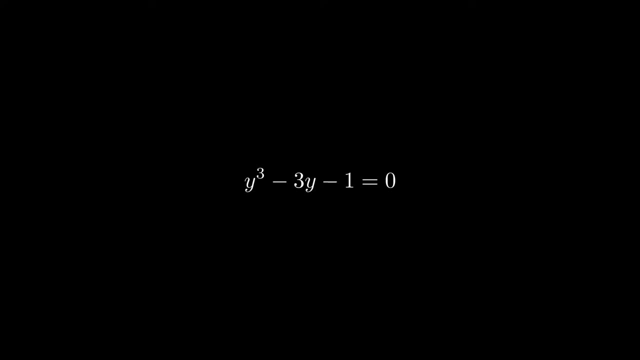 math shows that neither of these work, so this polynomial is not factorable over the rationals. Also, notice that 3 is not a power of 2, so finally, we can conclude that cosine of 20 degrees is not constructable, But this means that a 20 degree 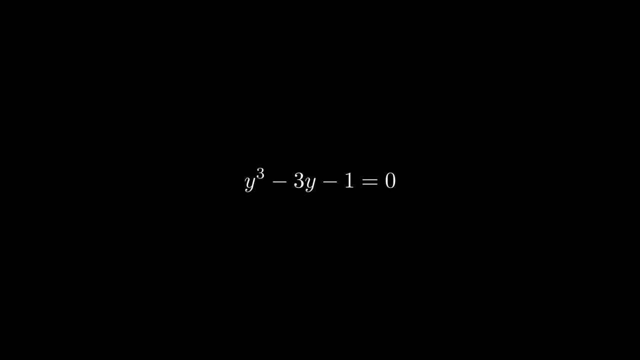 angle is not constructable either. so a 60 degree angle cannot be trisected. Just for a moment, let's peek into the world of ruler and compass constructions. If we're given an angle, then the problem of angle trisection has an easy, simple solution. 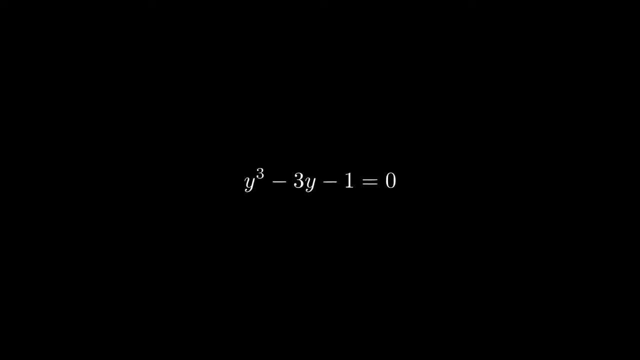 I'll substitute 2x for y, which will help us out in a bit. At this point, you might be asking yourself where we go from here. This is where abstract algebra comes in. Basically, any root to our polynomial is not constructable. 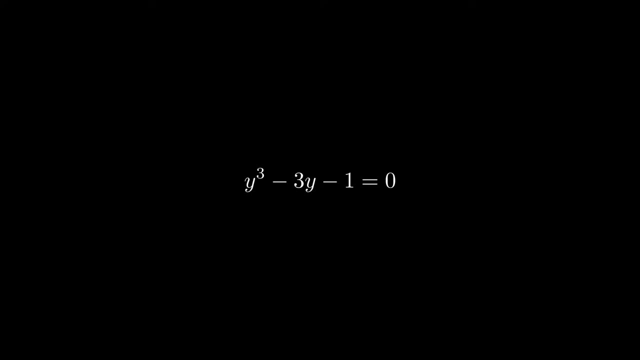 if we can't factor it with rational numbers, and its degree is not a power of 2.. To check whether this polynomial is factorable with rational numbers, all we have to do is use the rational root theorem. Our constant term is negative 1, and our leading coefficient is: 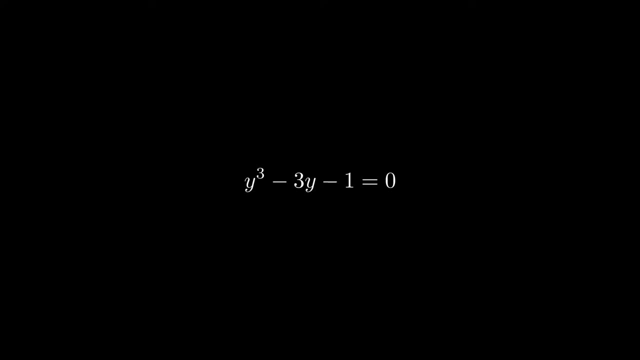 positive 1, so our only possible roots are positive 1 and negative 1.. Some quick mental math shows that neither of these work, so this polynomial is not factorable over the rationals. Also, notice that 3 is not a power of 2, so finally we can conclude that cosine of 20. 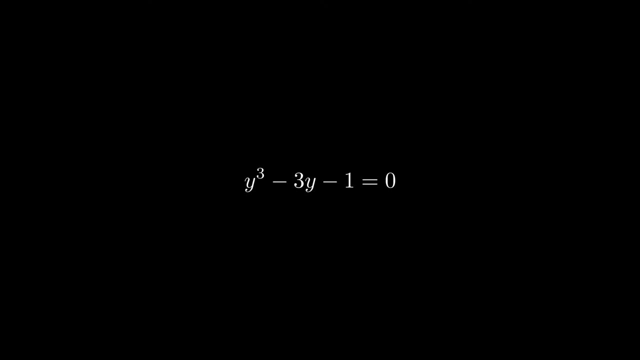 degrees is not constructable, But this means that a 20 degree angle is not constructable either. so a 60 degree angle cannot be trisected. Just for a moment, let's peek into the world of ruler and compass constructions. If we're given an angle, then the problem of angle trisection has an easy, simple solution. 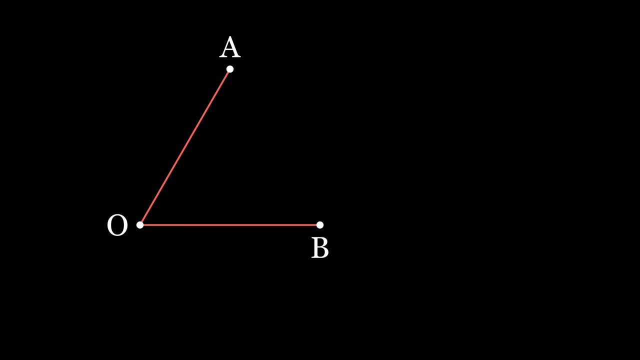 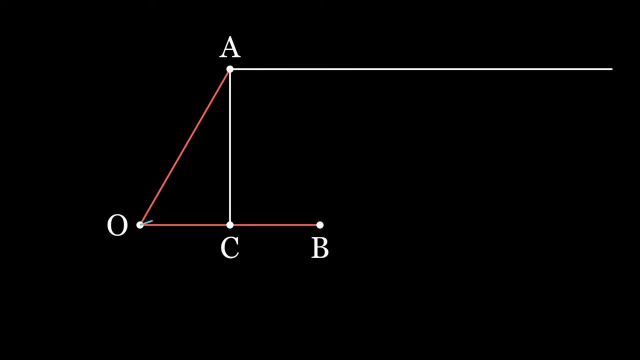 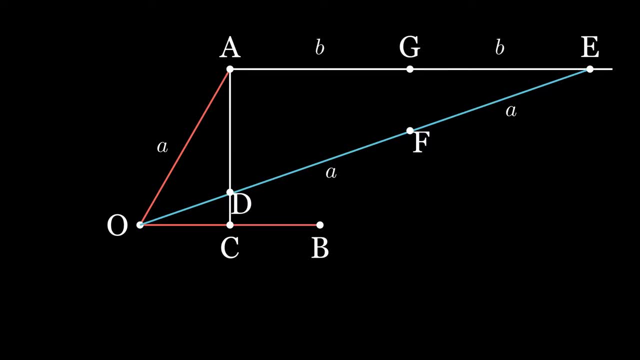 Next find G, the midpoint of AE, such that AG and GE have length little b. If we connect points G and F and A and F. If we connect points G and F and A and F, notice that by side-angle-side we had two congruent triangles. 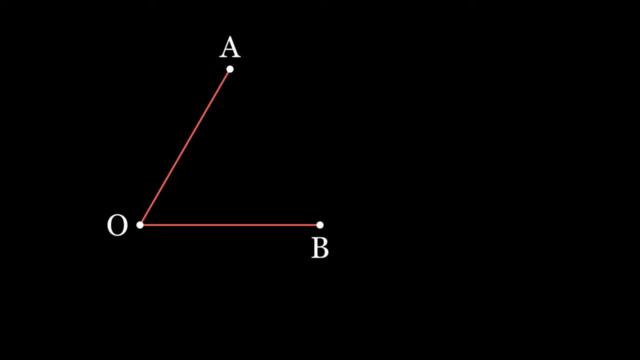 Say, we're given an angle which I'll call AOB. First drop a perpendicular from A to meet OB at C. Next draw a line to OB passing through A. Now, using a ruler, construct line OE such that DF and FE. 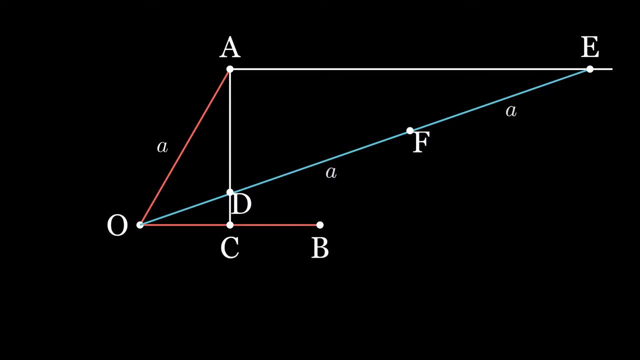 are equal in length to OA. For brevity I'll say OA has length a. Next find G, the midpoint of AE, such that AG and GE have length b If we connect points G and F and A and F. 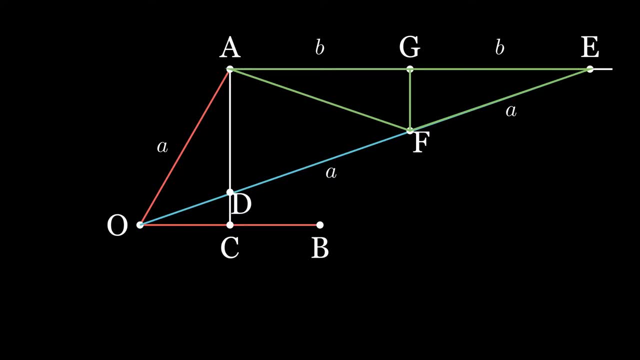 notice that by side, angle side, we have two congruent triangles: EFG and AFG. As a consequence, side AF also has length a. Now remember, we constructed the parallel line AE By alternate interior angles. we know that angle DOC, which I'll call alpha. 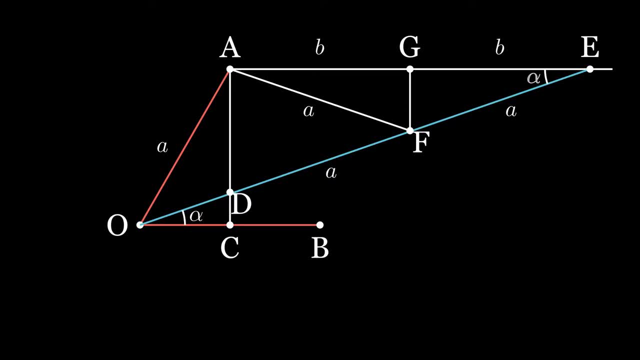 is congruent to angle GEF, which in turn is congruent to angle GAF, again by congruent triangles. Next, through a bit of algebra, we find that angle AFO is secretly 2A And as triangle, AOF is isosceles, that means that angle AOD is also 2A. 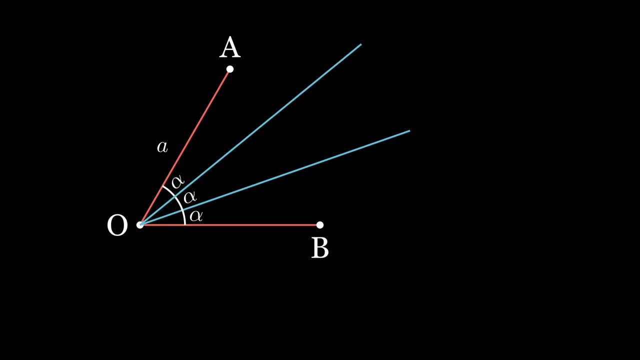 Finally, we can bisector angle AOD to get 2A's and thus the trisection of angle AOB is complete. Last we'll answer auric modelling to get an gives smallest angle and thatивar Billy's become 1 lbsЙ. 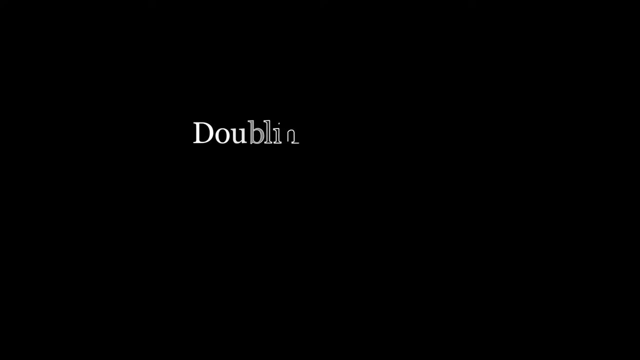 If both of this вопрос are answered correctly, we will have an equation in aでしょう. let's move on to our second problem: duplicating the cube. this one actually isn't too bad to recall say we have some cube. we want to show that it is not possible to construct a cube with twice. 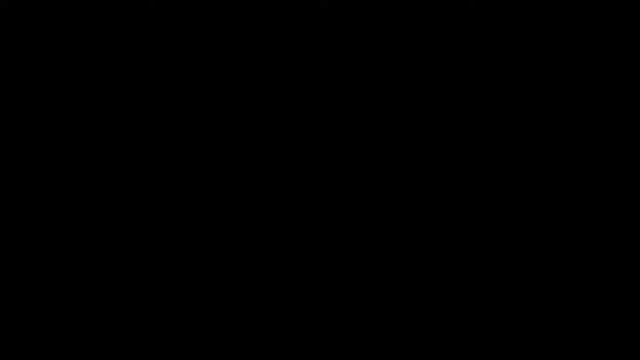 the volume of our original cube. for this problem, we'll just focus on the construction of the size of our cubes, as it's pretty straightforward to get the rest of the cube. let the side of our smaller cube be a and let the side of our bigger cube be b. what we want is for b cubed to be the. 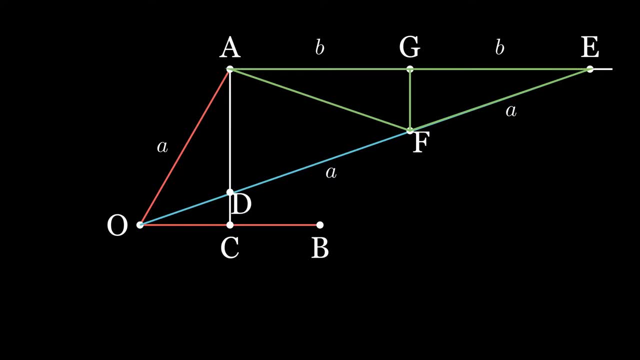 EFG and AFG. As a consequence, side AF also had length A. Now remember, we constructed the parallel line AE By alternate interior angles. we know that the angle DOC, which I'll call alpha, is congruent to the angle GEF, which in turn is congruent to the angle GAF. 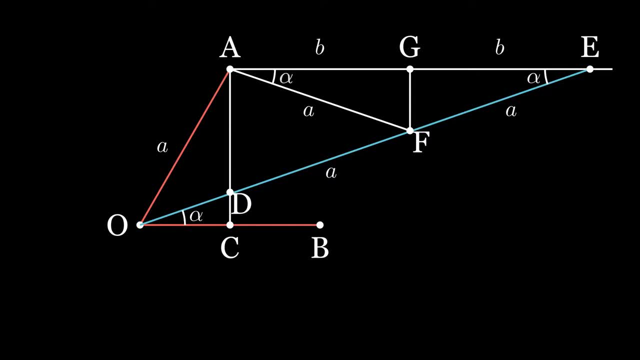 again by congruent triangles. Next, through a bit of algebra, we find that angle AFO is secretly 2 alpha and as triangle AOF is isosceles, that means that angle AOD is also 2 alpha. Finally, we can bisect angle AOD to get two alphas, and thus the trisection of angle. 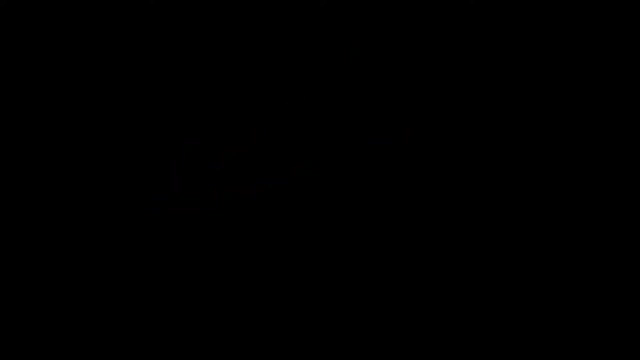 AOB is complete. Let's move on to our second problem: duplicating the cube. This one actually isn't too bad To recall say we have some cube. We want to show that it is not possible to construct a cube with twice the volume of 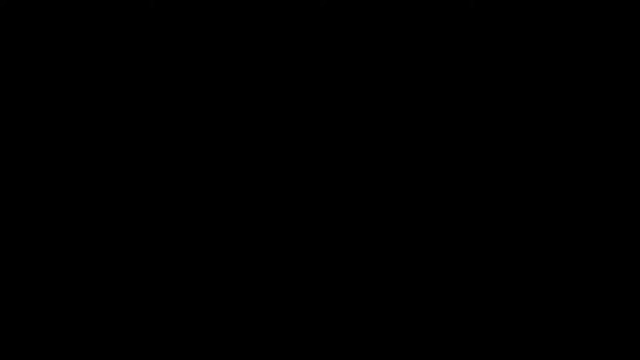 our original cube. For this problem, we'll just focus on the construction of the sides of our cubes, as it's pretty straightforward to get the rest of the cube: Let the side of our smaller cube be A and let the side of our bigger cube be B. but 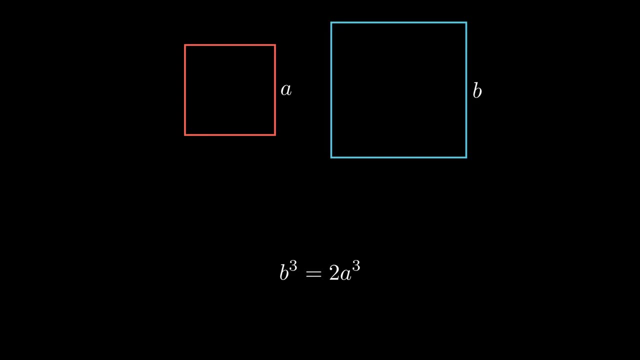 we want to duplicate the cube. We want the cube to be the same as 2 times A cubed. This means that B is equal to the cube root of 2 times A. To make the math a bit easier, let's let A equal 1, then B is just the cube root of. 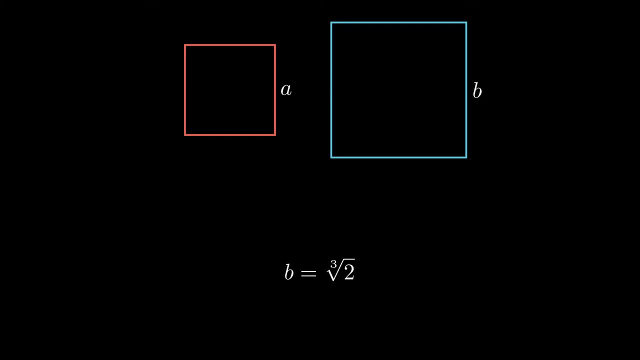 2. Now our problem of duplicating the cube boils down to whether or not the cube root of 2 is constructable. Similarly as before, let's consider the equation X cubed minus 2 times A cubed. The cube root of 2 is clearly a root of this equation. 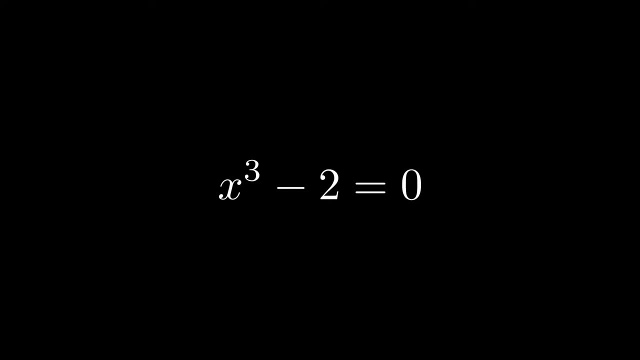 So, in order to determine whether it's constructable, we have to figure out whether or not we can factor this polynomial over the rationals. Another application of the rational root theorem quickly shows us that we can't do this. And as the degree of our polynomial isn't a power of 2,, it follows that the cube root 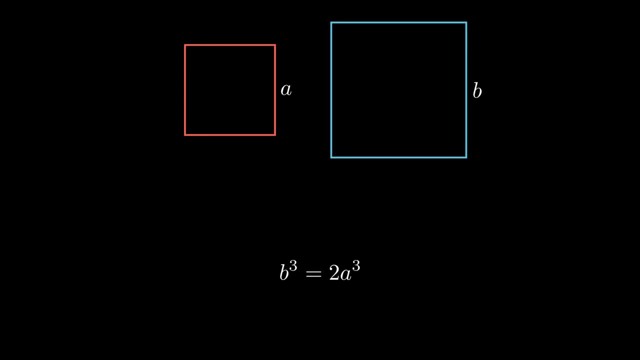 same as two times a cubed. this means that b is equal to the cube root of two times a. to make the math a bit easier, let's let a equal one. then b is just the cube root of two. now our problem of duplicating the cube boils down to whether or not the cube root of two is constructible. 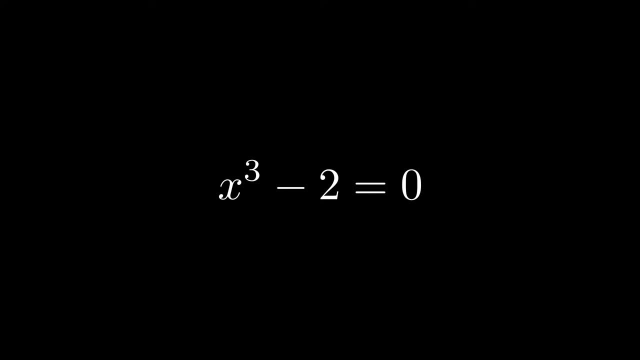 similarly as before, let's consider the equation x cubed minus two equals zero. the cube root of two is clearly a root of this equation, so in order to determine whether it's constructible, we have to figure out whether or not we can factor this polynomial over the rationals. 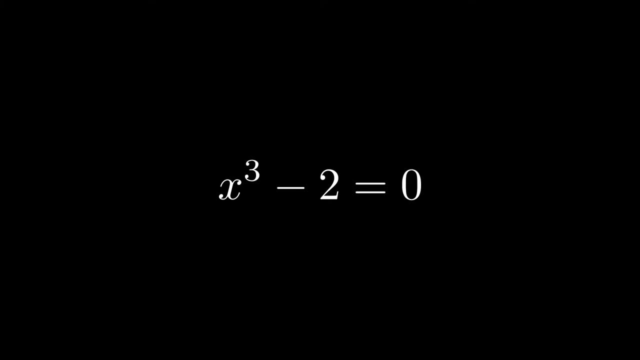 another application of the rational root theorem quickly shows us that we can't do this, as the degree of our polynomial isn't a power of two. it follows that the cube root of two is not constructible as well. finally, to wrap it up, let's look at my favorite problem: squaring the 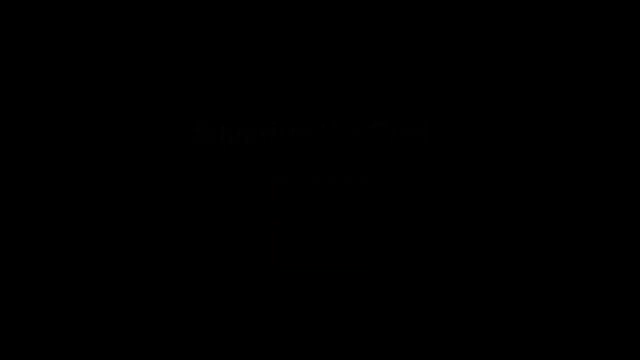 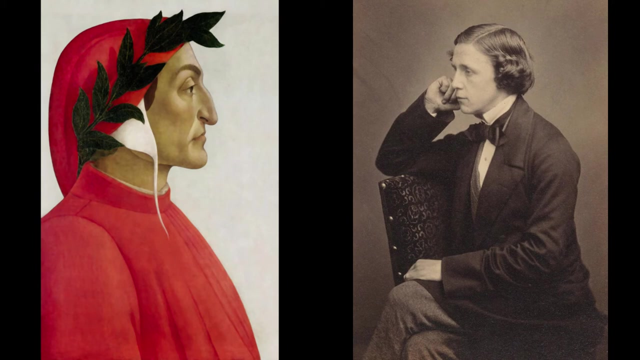 circle. firstly, i just want to say that this problem in particular is quite infamous for its difficulty. the proof for its impossibility took more than 2 000 years. even dante of dante's inferno and lewis carroll of alice's adventures in wonderland knew of the problem, and today it's seen. 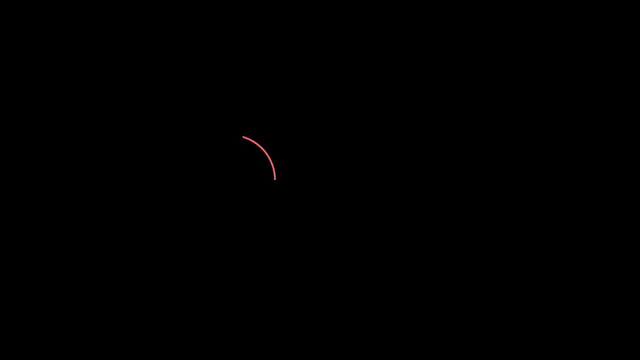 as a metaphor for attempting the impossible. suppose we have some circle with radius r. we know that its area is just pi times the radius squared. and suppose we have a square with side length s, then its area is simply s squared. what we want is for these two areas to be the same, so through a bit of algebra we can find that s. 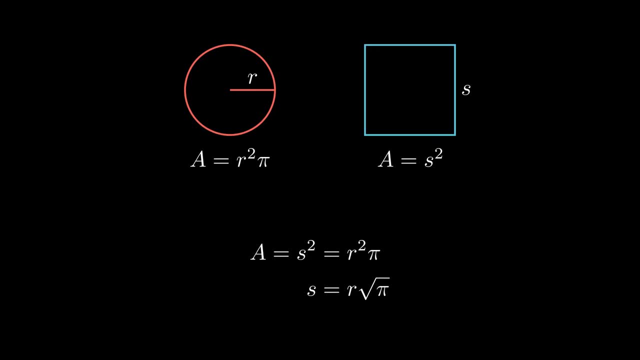 has to be equal to r times the square root of pi. now keep in mind, r could be any number, so to make the math a bit easier, let's let it be one. what we get is: s is equal to the square root of pi. again we must ask ourselves: is the square root of pi constructable? i don't think it's much of. 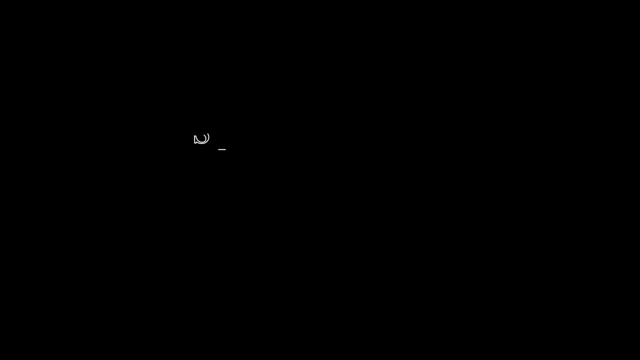 of 2 is not constructable as well. Finally, to wrap it up, Let's look at my favorite problem: squaring the circle. Firstly, I just want to say that this problem in particular is quite infamous for its difficulty. The proof for its impossibility took more than 2000 years. 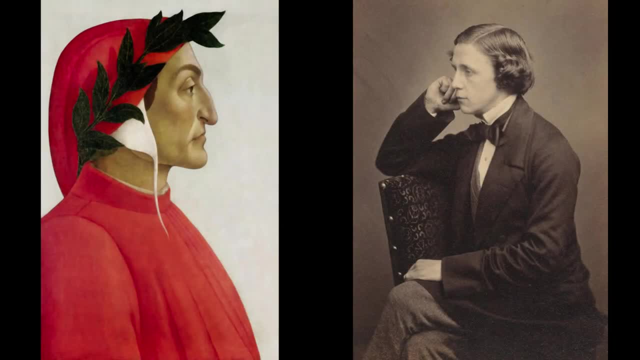 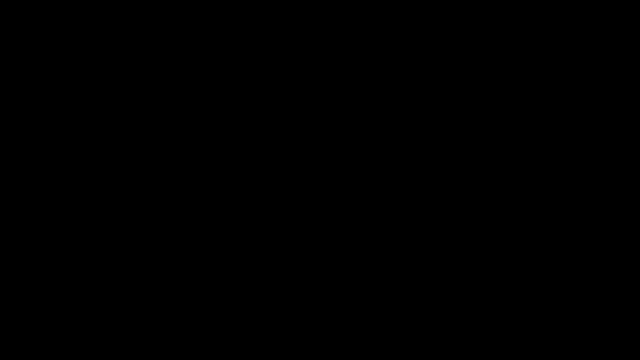 Even Dante of Dante's Inferno and Lewis Carroll of Alice's Adventures in Wonderland knew of the problem, and today it's seen as a metaphor for attempting the impossible. Suppose we have some circle with radius r. We know that it's a circle. 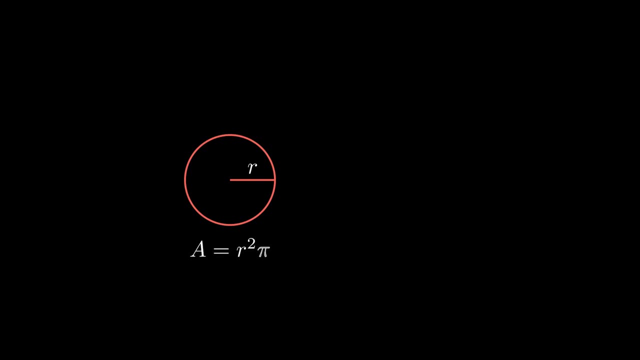 Suppose we have some circle with radius r. Suppose we have some circle with radius r And now it's triggered by부, Does this mean that that square over that area is just pi times the radius squared? And suppose we have a square with side length s, then its area is simply s squared. 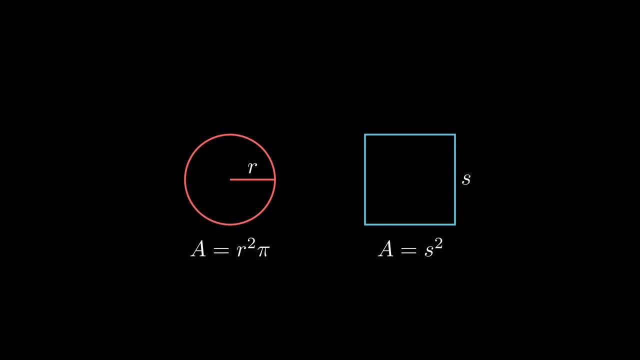 What we want is for these two areas to be the same. So through a bit of algebra, we can find that r is equal to r times square root of pi. Keep in mind r could be any number. so to make the math a bit easier, students, let's. 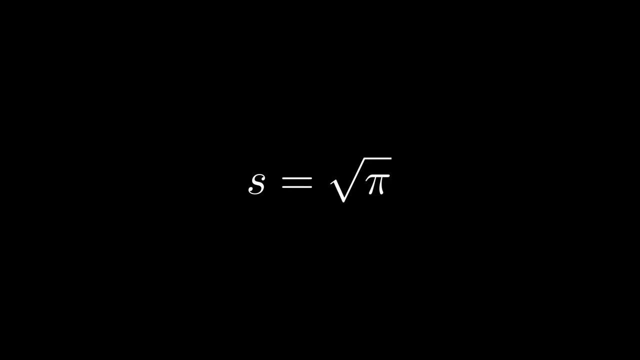 let it be 1. to the square root of pi. Again, we must ask ourselves: is the square root of pi constructible? I don't think it's much of a stretch to say that if the square root of pi is constructible, 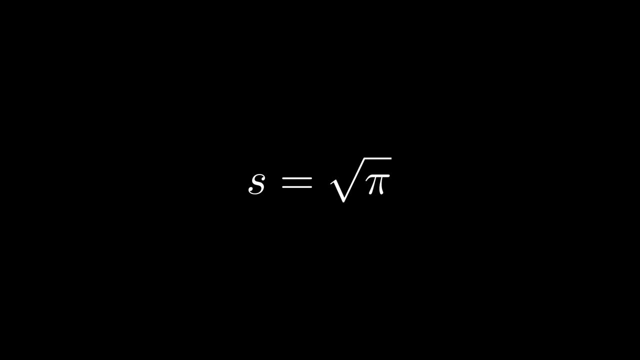 then pi must be constructible too. However, there's a remarkable result of number theory that dates back to Linman of the 19th century, which says otherwise. Essentially, Linman proved that pi is transcendental, which implies that pi cannot be constructible. 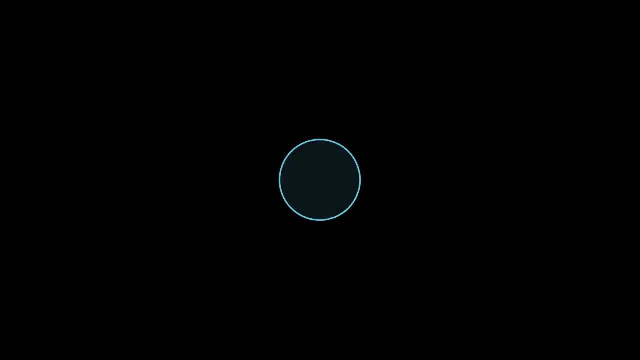 Now that you're an experienced geometer, you might wonder why mathematicians decide to use their time by trying to solve these problems in the first place. After all, it's not like your barista is ever going to ask you to square a circle, so why bother? Well, 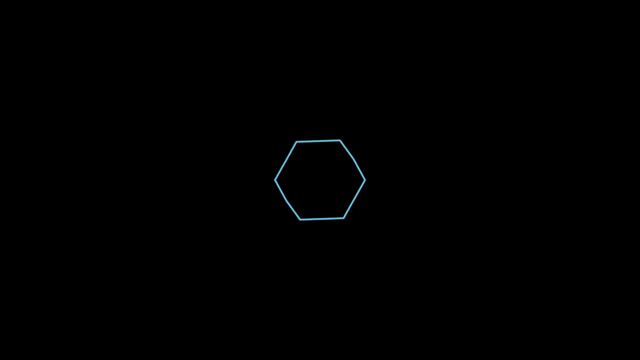 it all comes down to a common theme that frequently comes across any seemingly difficult math problem: abstraction. By making the same problem as the previous problem, we get to the point where divide by square. By making the same problem as the previous problem, we get to the point where